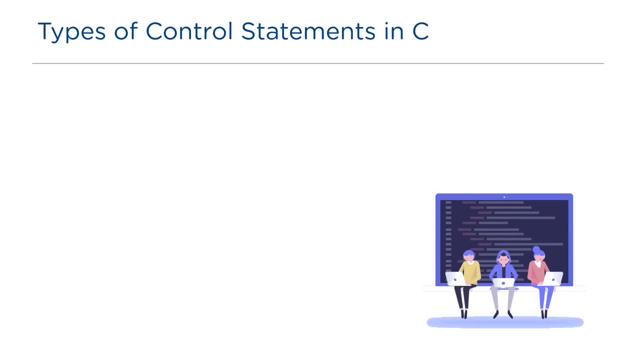 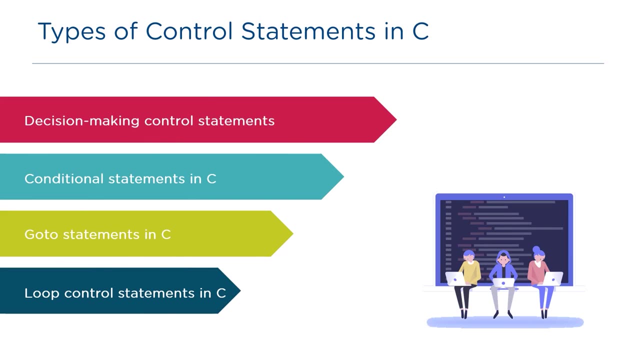 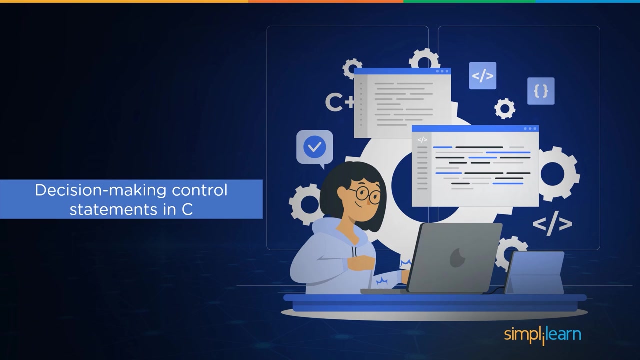 of control statements in C. First up we have decision making control statements, Then we have conditional statements And finally go to statements and loop control statements. First let us understand all the decision making control statements in C First let 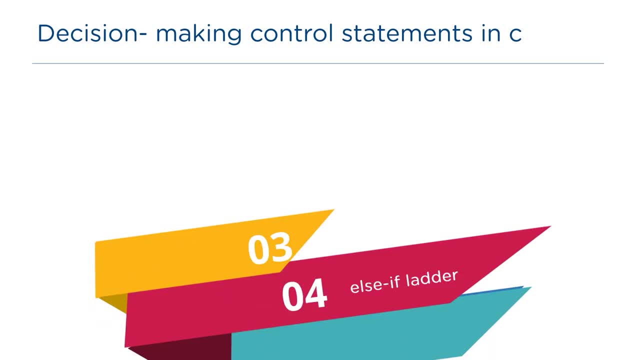 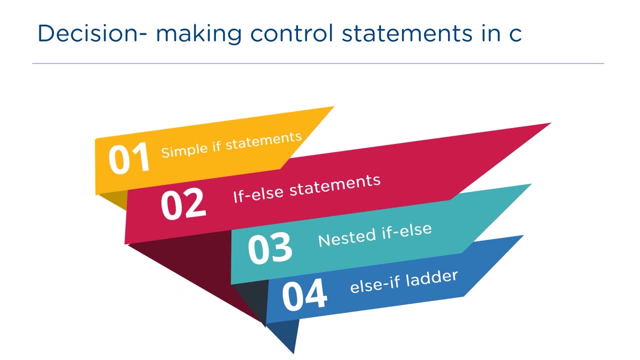 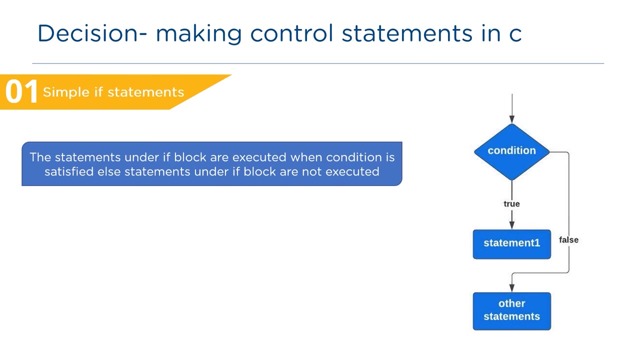 us find position making control statements. Decision making control statements are Simple: IF, IF-WELLS, nested If-Wells statements and Else if ladder. Let us go through them in detail. Now let us have a look at the Simple if statements. When you look at the flow chart, it is very clear that the if first evaluates the if condition. 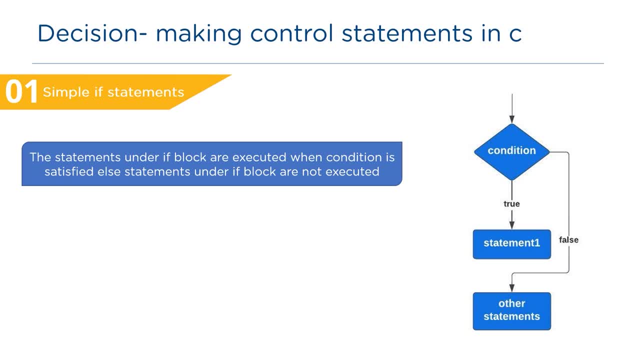 And if the condition is true, the statements under if will be executed. Else other statements outside the if will be executed. and the syntax of simple if is if condition, followed by statement inside the curly brackets. now let's execute the simple program using if statements, if getting. 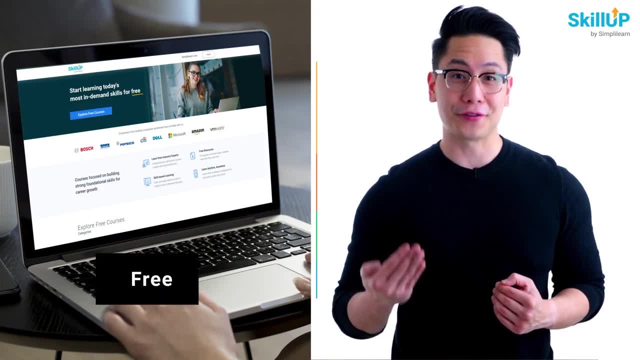 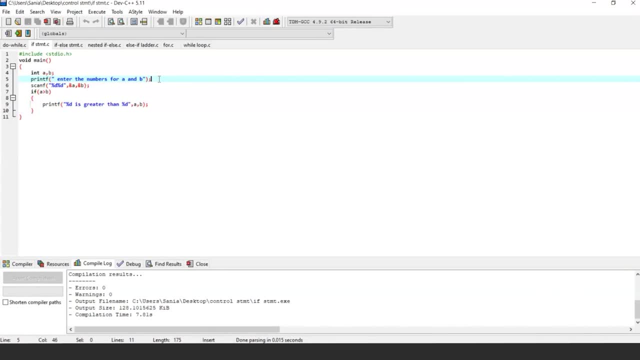 your learning started is half the battle. what if you could do that for free? visit. scale up by simply learn. click on the link in the description to know more. in this particular program, based on simple if statement, it asked user to enter value for a and b and it checks the condition a greater. 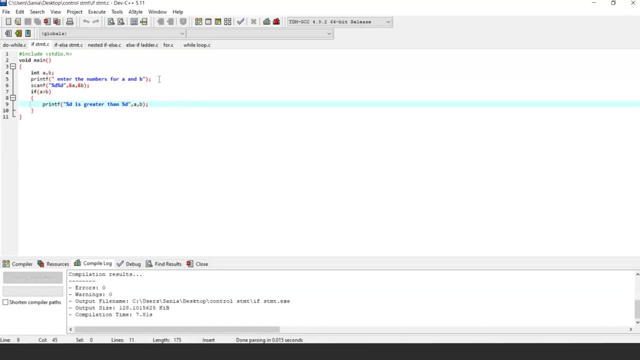 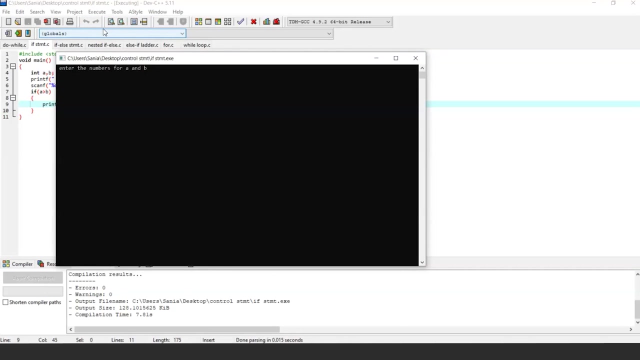 than b, and if a is greater than b, it prints the statement a is greater than b. in case a is not greater than b, it will not print anything. now let's run it. enter the numbers for a and b, let's enter 10 and 5, and the output is: 10 is greater than 5. 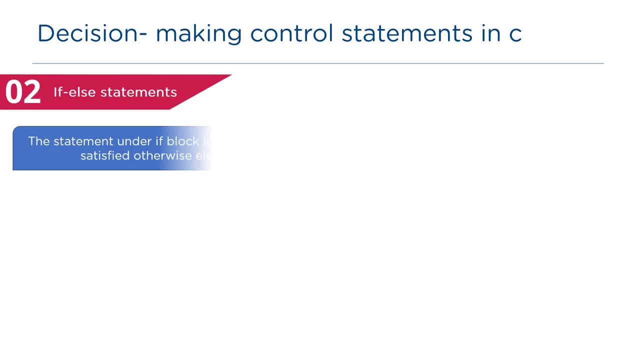 next, if in statements. in this it evaluates the condition and if the condition is true, the statements under if will be executed. otherwise, these statements under else will be executed and followed by other statements. syntax of if a statement is: if condition. statement 1 is statement 2. let's understand the if-else statement with the help of an example program. 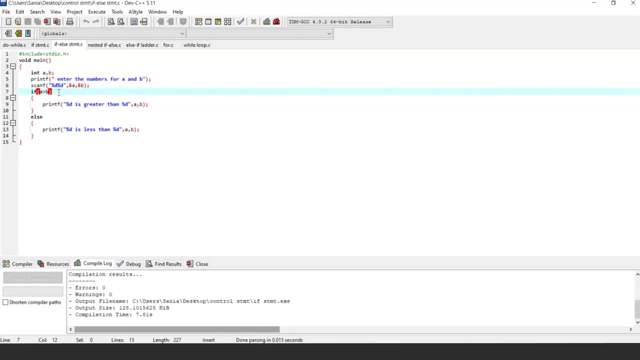 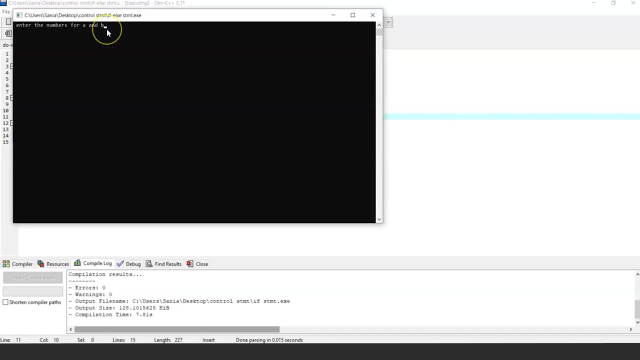 this particular program is based on if-else statement, as i discussed before. it checks the if condition and if the condition is satisfied, it will print the statement under if block. otherwise it will print the statements under else block. let's run it. enter the numbers for a and b. 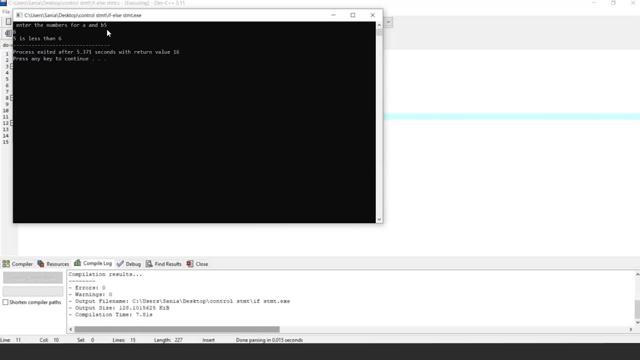 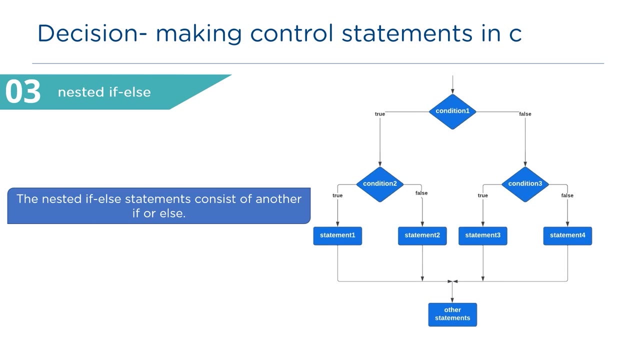 so, as you all can see the output, the value of a is not greater than b. that's why this statement under else block is executed. next we have nested if-else statement. the nested effects statements consist of another if or else. let us understand nested equal statements with the help of syntax. 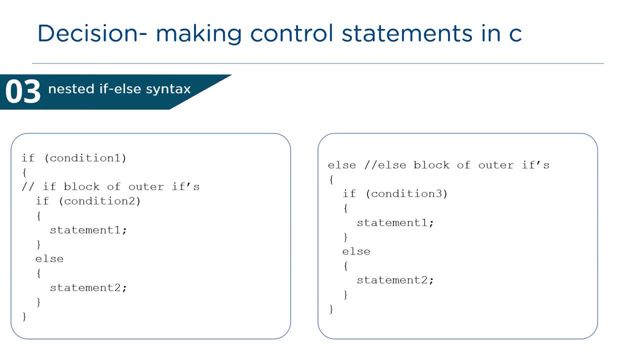 this consists of another event statement inside the outer if block and another if-else. if- deneralize is executed as a non-existent element. It represents different types of properties, ie in other words if and b as every other, a parent's statement. this consists of another if-else statement inside the outer if- block and another if- else in the other, a parent's block. 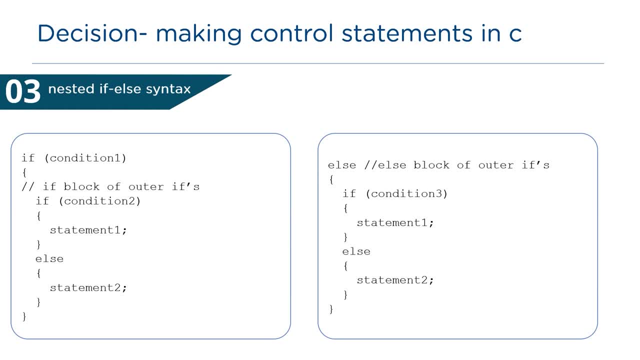 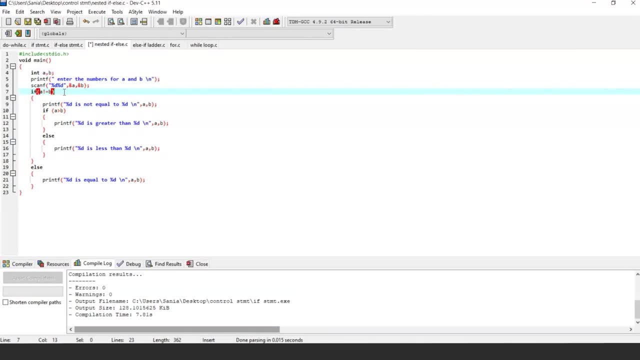 This consists of another if-else statement�: chassis slot-out, ding-over- if aspect fingers. another if-else inside the outer-else block. Let's understand by an example. This program is based on nested if-else. This is an outer-if block and it consists of: 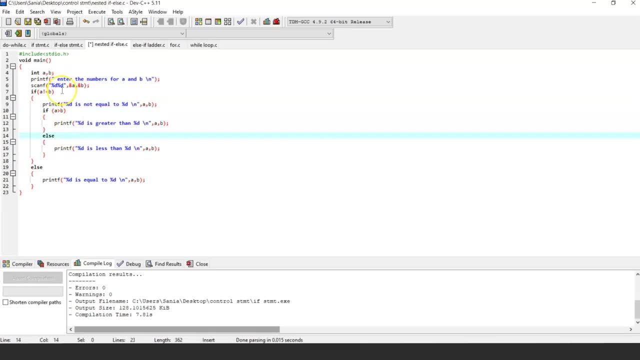 another, if and else. It first checks the condition of outer-if, and if the condition is not satisfied, then it checks the inner-if condition. Even if that condition is not satisfied, it executes the statement under else block In case even that condition is not satisfied. 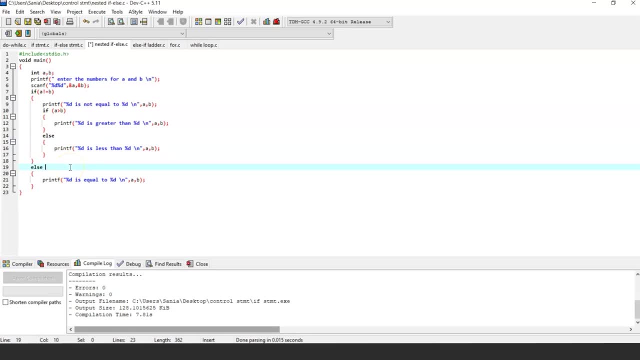 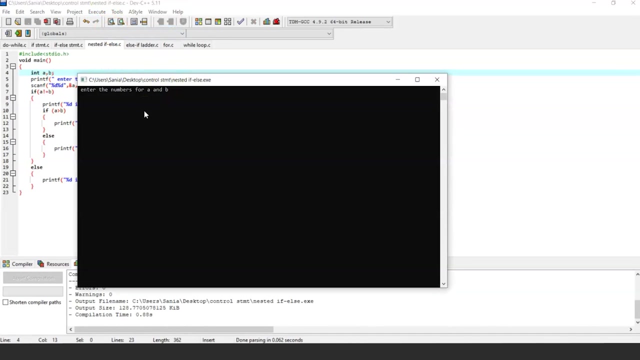 it comes outside the outer-if block and executes the statements under outer-if-else block. Let's run it. Enter the numbers for a and b, Then enter. As you can see, the value of a and b are same. It has printed statement. 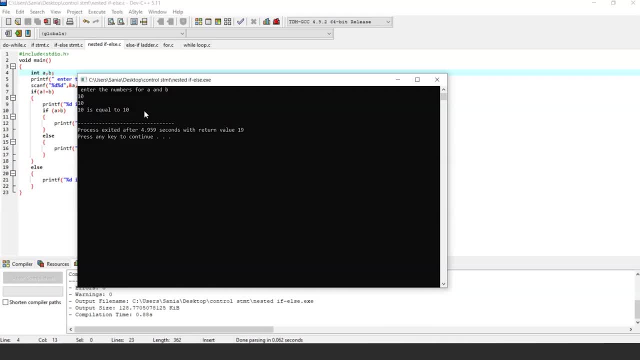 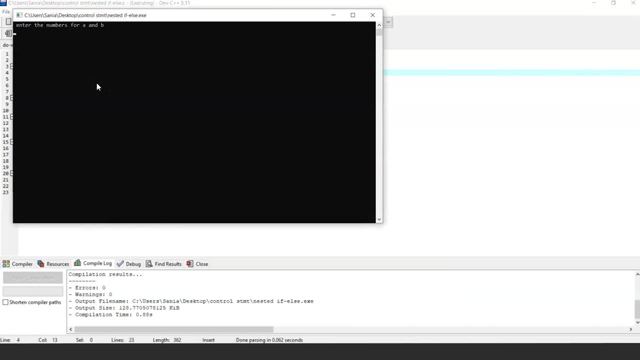 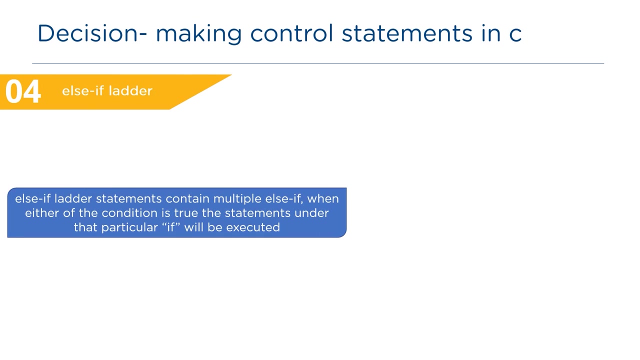 under outer-else block. Now let's enter different values for a and b and check the output. So since a is not equal to b and a is greater than b, the output is printed successfully. Next: else-if ladder. Else-if ladder statements contain multiple else-if. 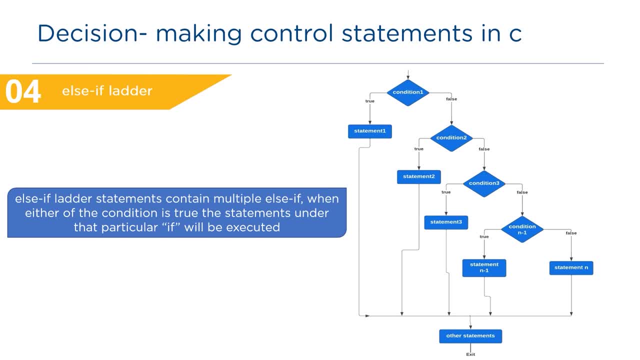 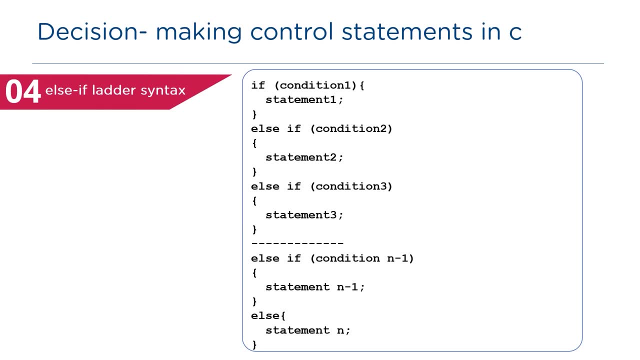 Else-if ladder statements contain multiple else-if. Else-if ladder statements contain multiple else-if. If the condition is true, the statements under that particular if will be executed. Otherwise, the statements under the else block will be executed. The syntax is if condition and followed by multiple else-if. 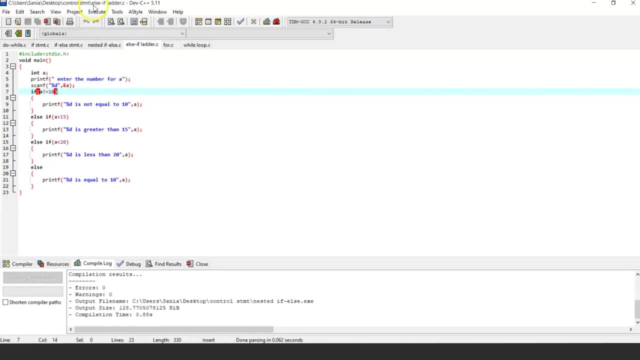 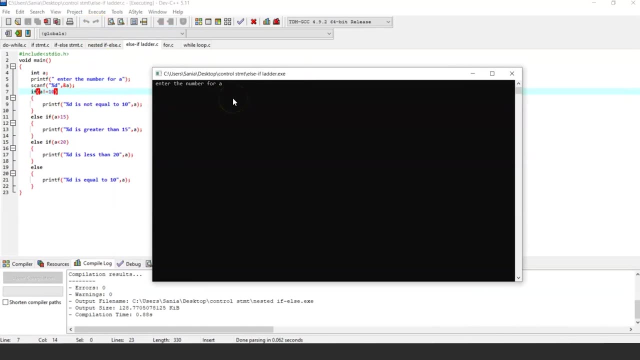 So now let's execute the program using an else-if ladder. Enter the number for a, Let's enter 10.. So it checks the condition a not equal to 10.. Since the condition is not satisfied, it checks the next if condition. 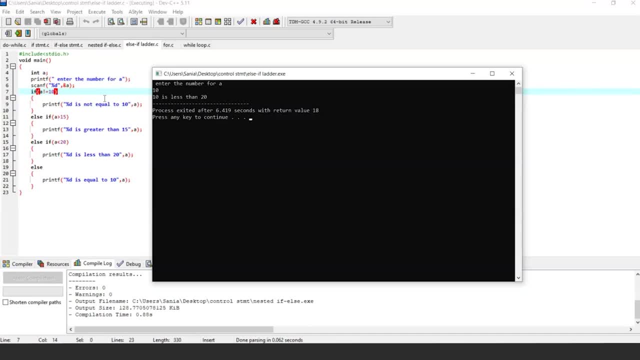 Since a is not greater than 15, it checks another if condition And the condition a less than 20- is satisfied And the output is 10 is less than 20.. Now let's have a look at the control statements in C. 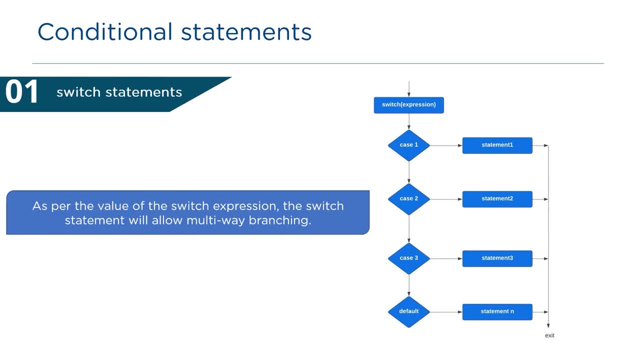 As per the value of switch expression. the switch statement will allow multi-way branching Depending on the expression. the control is transferred to that particular case label and execute the statements under it. If none of the cases are matched with the switch expression, then the default statement is executed. 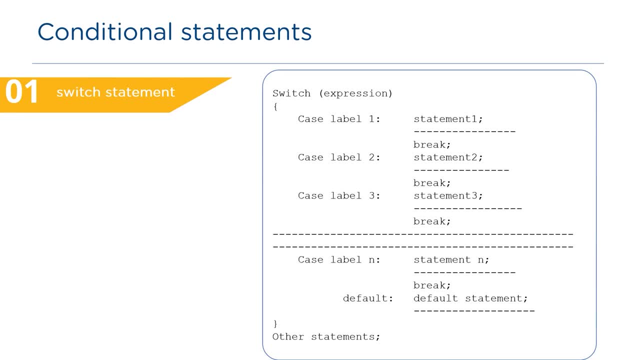 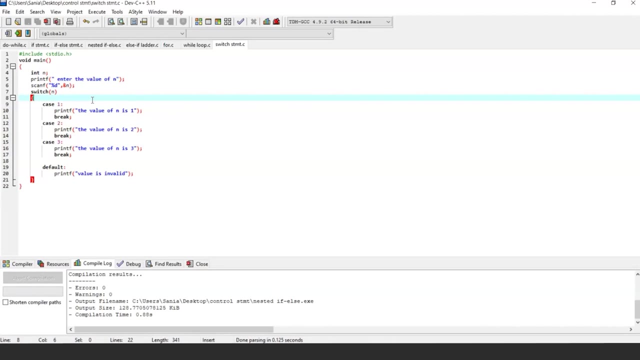 Syntax of switch statement is switch expression and inside the curly brackets, multiple case labels and at the end, default statement. Let's execute program based on switch statement. So in this particular program, if the expression of switch matches with any of the case label, 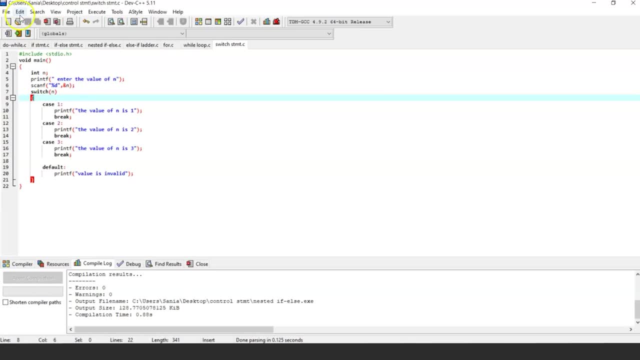 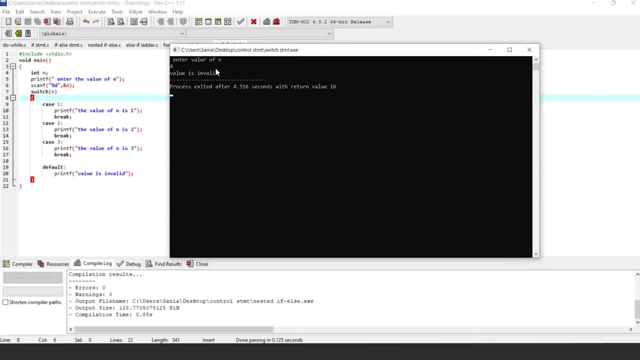 then it will execute the statements under it. Now let's run the program, Enter value of n, Let's enter four, And the output is: value is invalid. It's because, since the value of n is not matched with any of the case label. 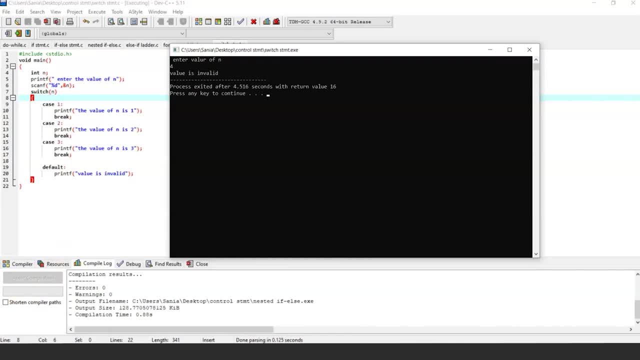 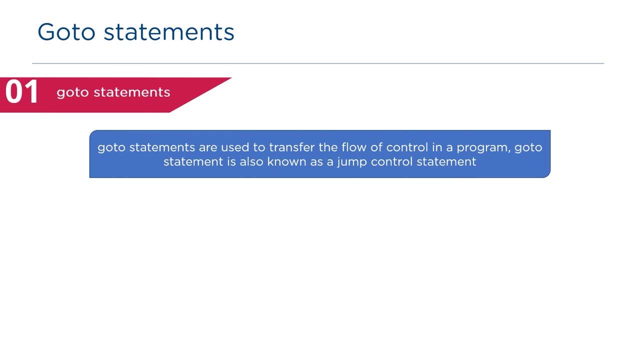 it has print the default statement. Now let's have a look at goto statements. Goto statements are used to transfer the flow of control in a program. Goto statement is also known as jump control statements because it is used to jump to the specified part of the program. 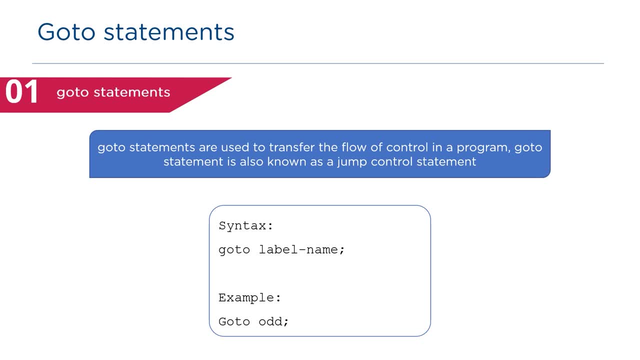 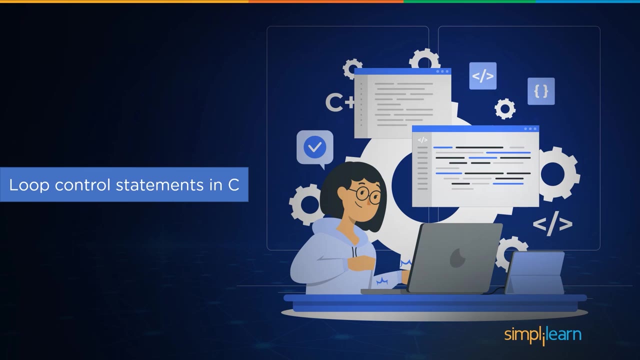 The syntax is goto label name and semicolon Label in goto statement is a name used to direct the branch to a specified point in the program. In the example, label name is odd. Next we have loop control statements in C. 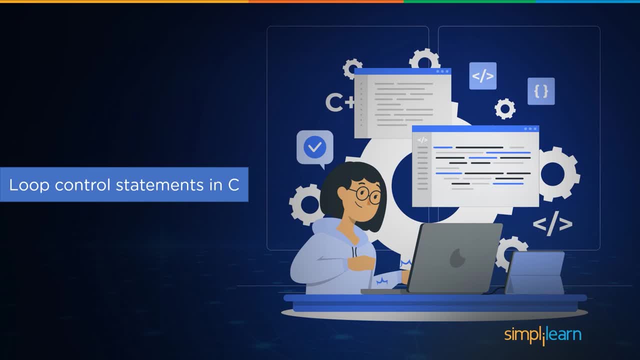 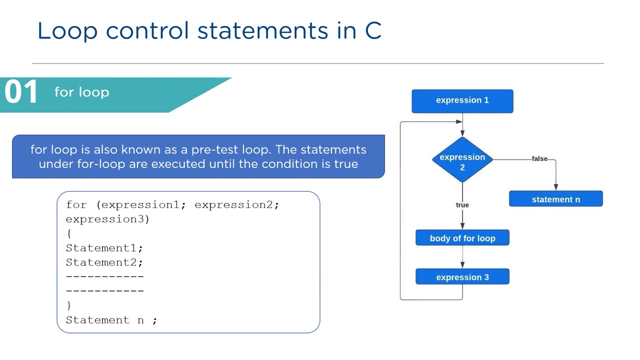 In loop control statements we have for loop, while loop and do while loop. Let us go through them in detail. For loop is also known as pre-test loop From the following syntax expression: one is an initialization expression. two is the conditional expression. 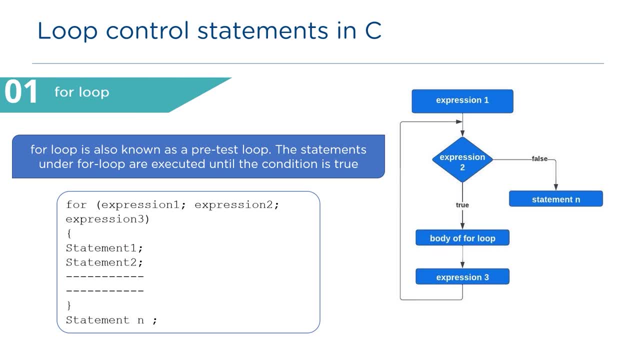 and expression. three is an updation. The variables can be initialized in the for loop statement itself. You might get a clear idea of using for loop when you look at the flow chart. In the for loop expression, one is used to initialize the variable. 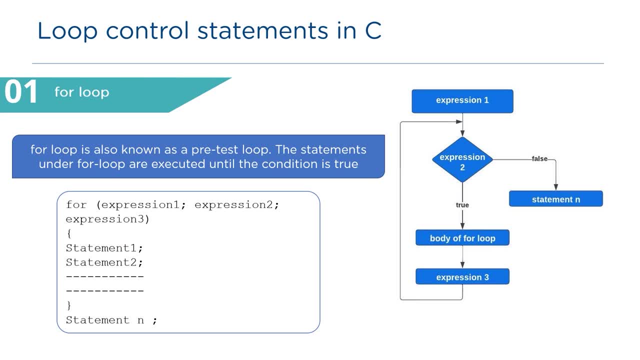 expression two is evaluated, and if the condition is true, then the body of for loop will be executed, And then the statements under expression three will be executed. This process is repeated as long as the for loop condition is true. Once the condition is false, 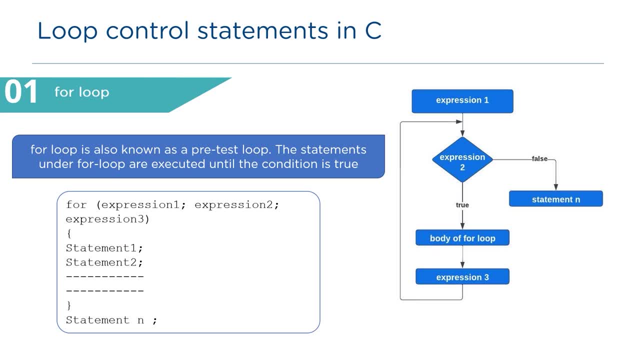 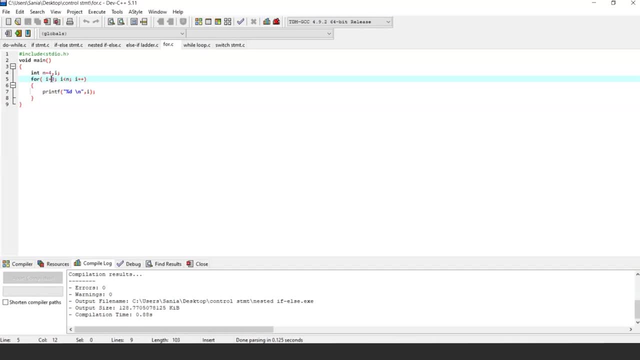 control will return to the statements following the for loop and execute those statements. Let's see the example. In the for loop, the variable i is initialized to zero and expression two is the condition, that is, i less than n, and then the updation. 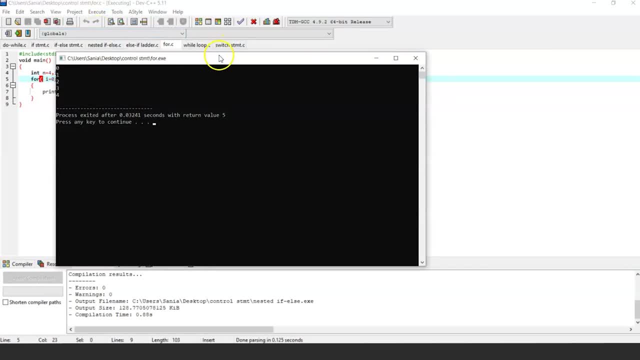 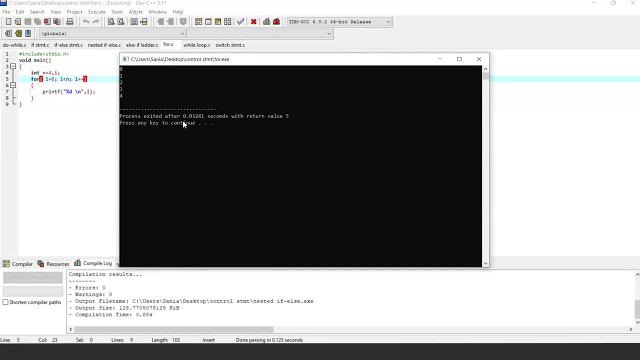 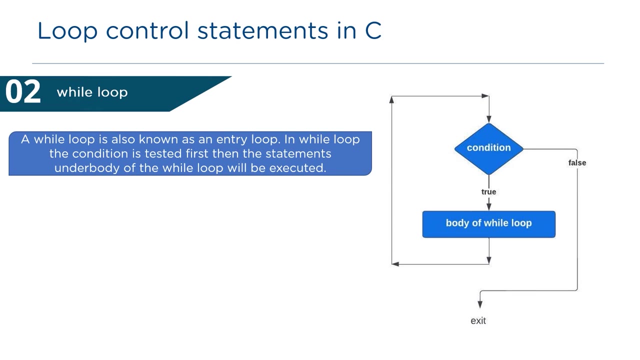 Let's run it. As you can see the output: the value of i is printed until the condition is false, Let's run it Up. next we have a while loop. A while loop is also known as an entry loop, because in a while loop the condition is tested first. 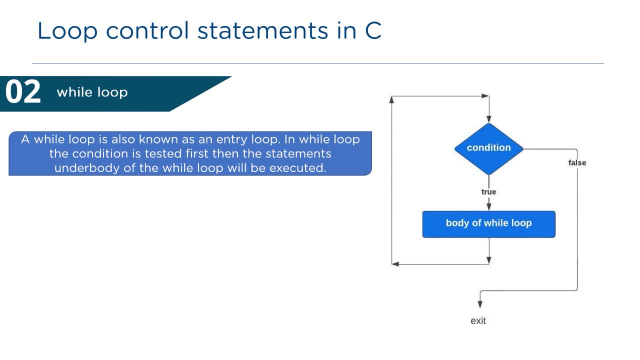 then the statements under body of the while loop will be executed. If the while loop condition is false for the first time itself, then the statements under the while loop will not be executed even once. Let's have a look at the syntax of a while loop. 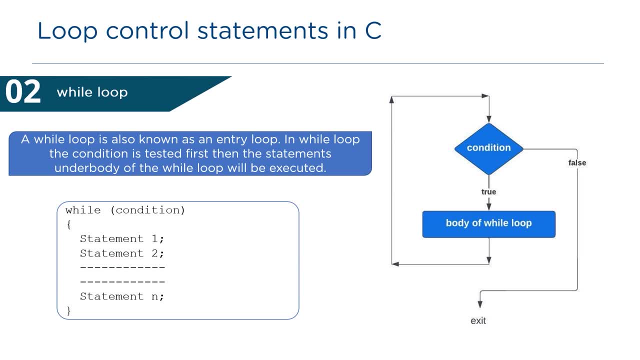 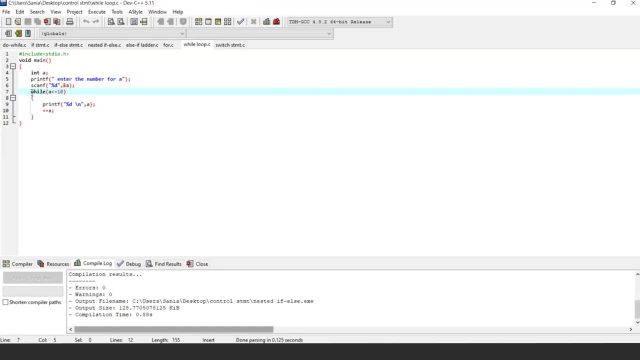 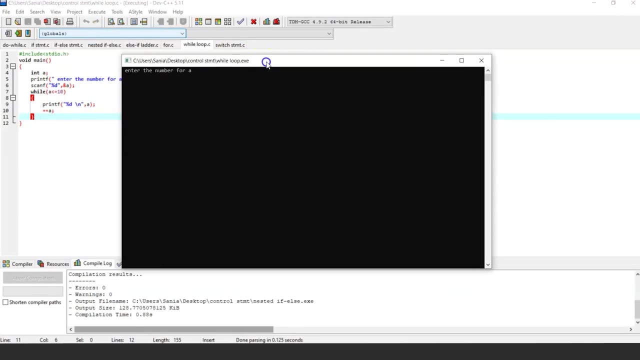 While condition and inside the curly brackets we have statements. Let's execute the program using while loop. So here it first checks the while condition and then prints the statement. Let's run it. Enter the number for a. Let's enter five. 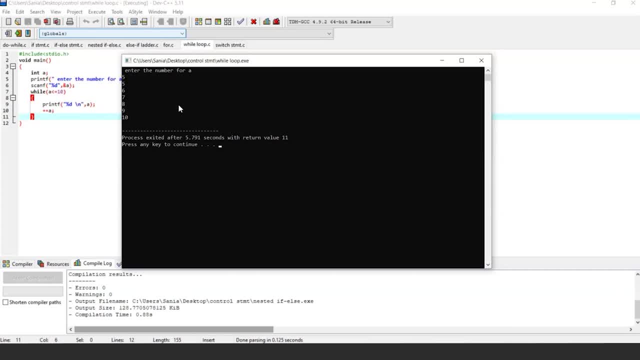 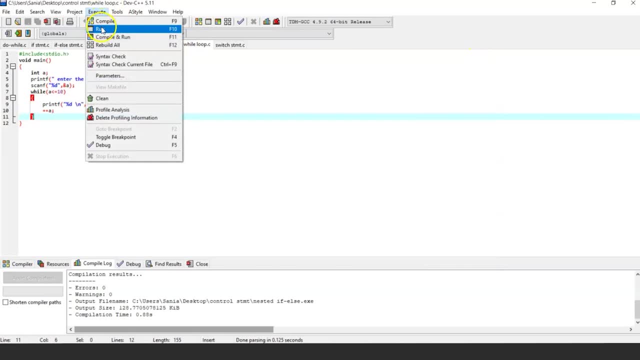 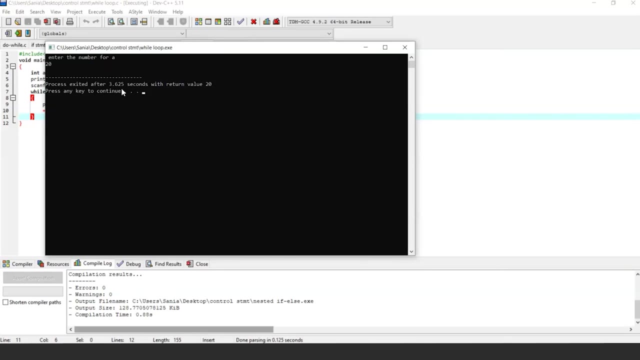 So, since the condition is satisfied, it has executed statements under the while loop. Now let us try to enter different value for a. Let's run it. Let's enter 20.. Since the condition is not satisfied, that is, 20 is not less than or equal to 10,.